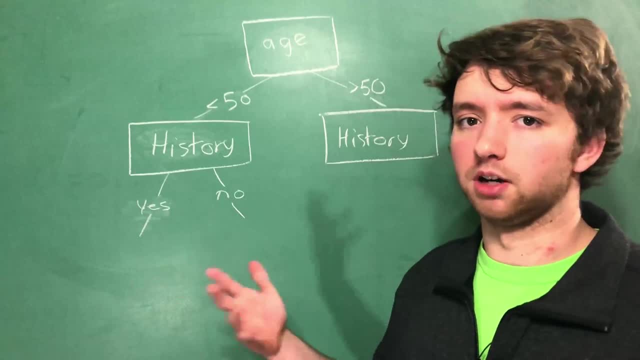 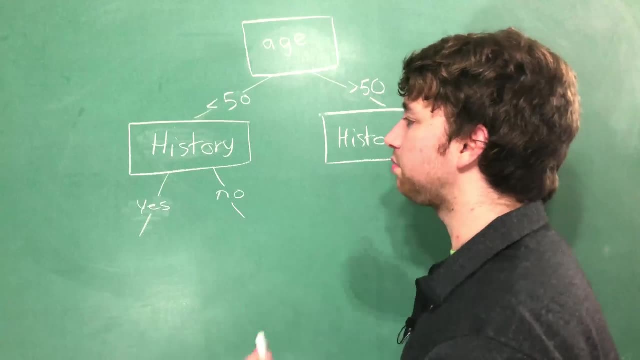 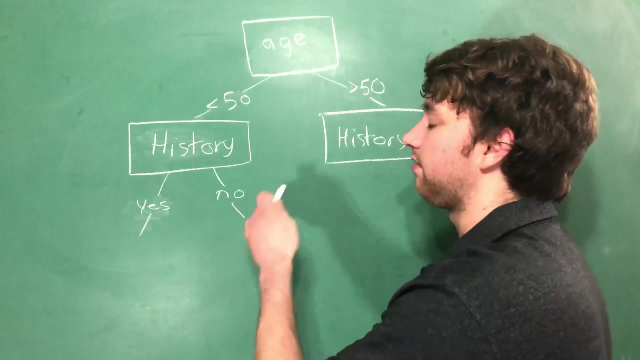 you had a family history of disease, or specifically diabetes. Well, yeah, I did So now I'm going to ask you a new question to get more detailed responses. At some point we're going to come to a conclusion. For example, using our historical data, everyone under 50 who does not have 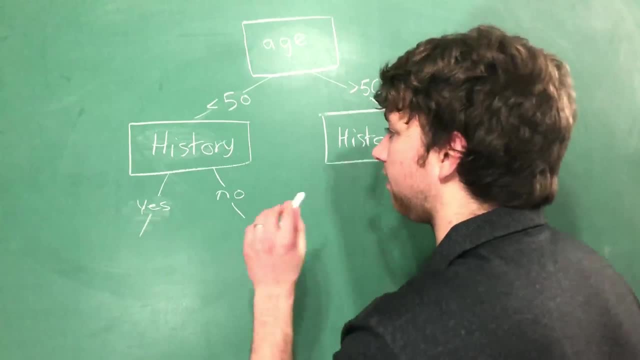 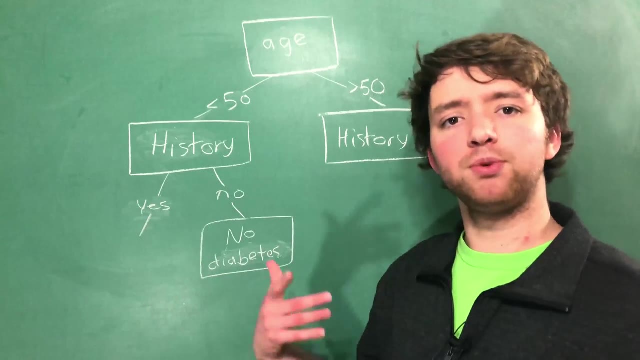 a family history of diabetes might have no chance of diabetes. Yes, on the other hand, might be more of a concern because, well, they had a family history. So maybe we have to ask another question. So the next question might be weight, And we could branch in three. 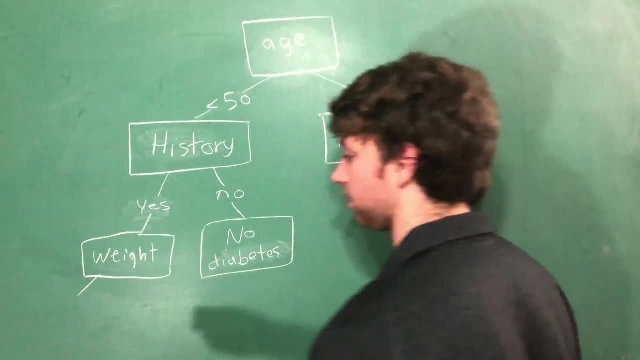 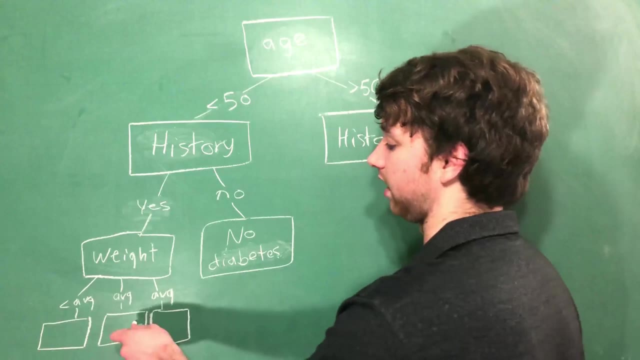 for this one We could say less than average, average and above average, And using our data, we might find that people who are less than average in this situation do not have diabetes. Those who are average do not have diabetes, But those who are greater. 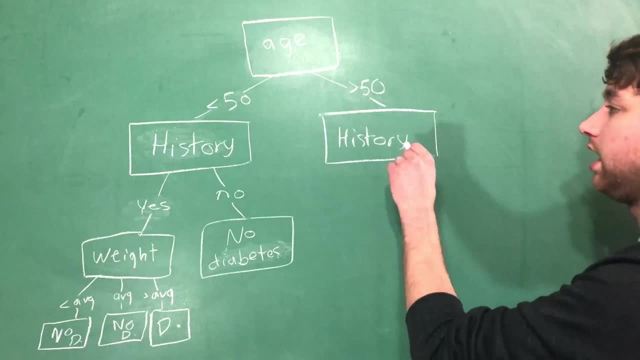 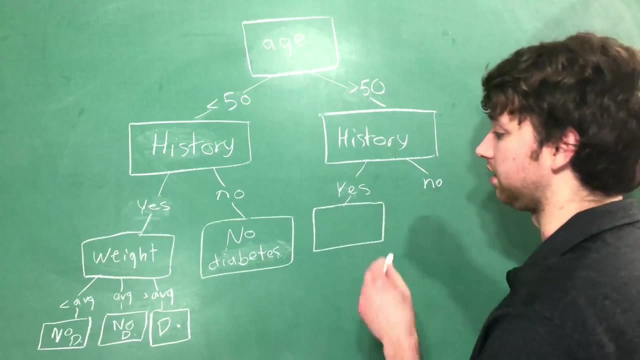 than average, do have diabetes. Now let's go over to this end history. Do you have a family history of diabetes? So those who are over 50 and have a history of family diabetes, well, our data might show that, yes, they're going to have diabetes. And those who do not? 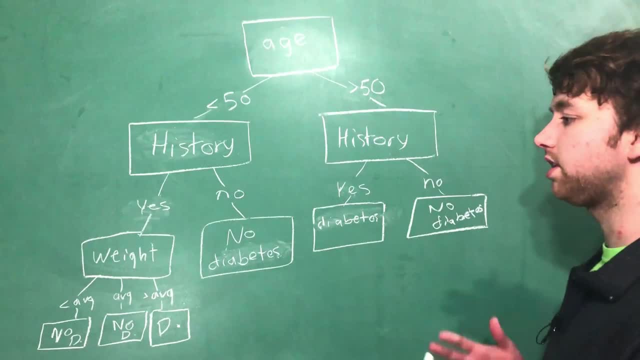 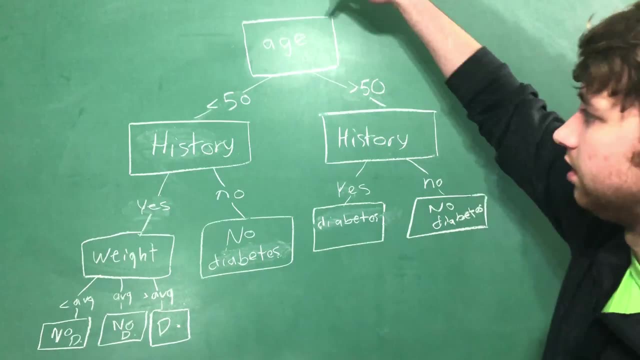 have a family history, we'll just say they don't have diabetes. So this here might represent our entire data set. This is our model of reality. So you go into the doctor's office. you can think of being classified in these different groups, down to where we get to. 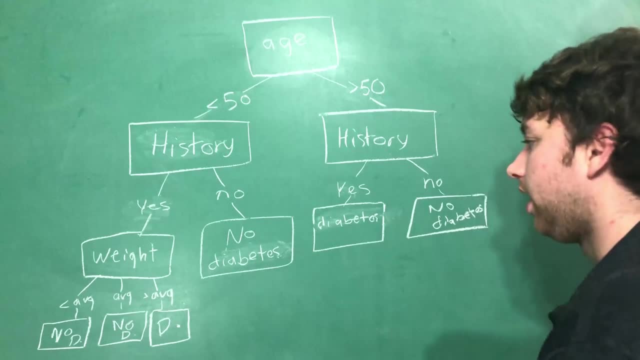 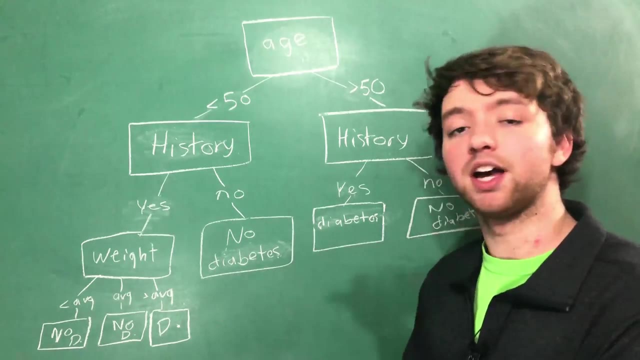 the final point, which is figuring out the target feature. As you can notice, all of the leaf nodes are a value for the target feature, And that target feature is whether you have diabetes or not. That is the point of the decision tree. We're splitting our 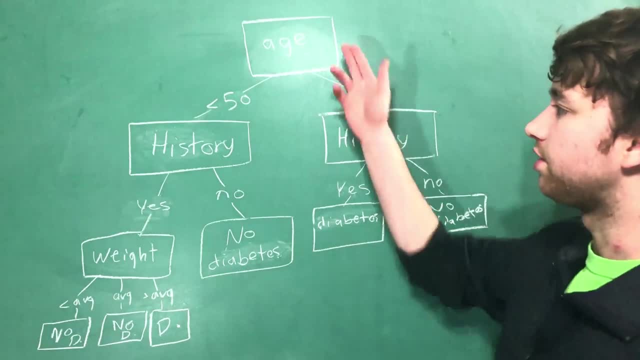 data until we get to the end result. So you go to the doctors and you're less than 50. They ask you: oh, do you have a family history of disease? You say yes. What's your weight? Oh, you're above average. 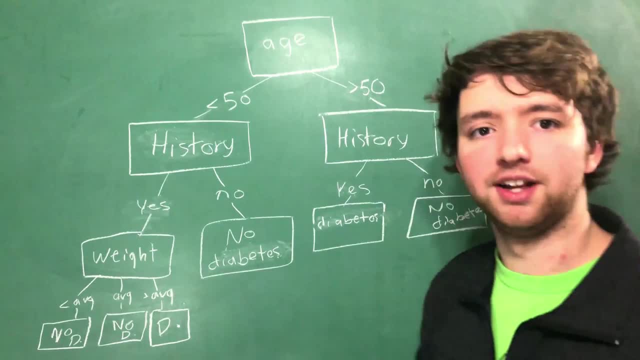 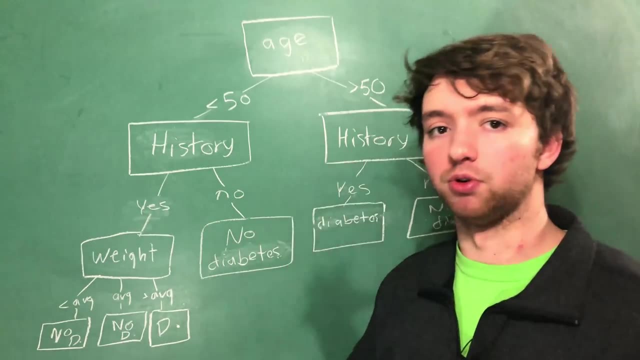 And you're going to have diabetes. Simple example, not entirely realistic, But once again, you want to remember that these are going to be groups of people that determine this kind of thing. So to illustrate, let's say we have a huge data set of like 10 people.